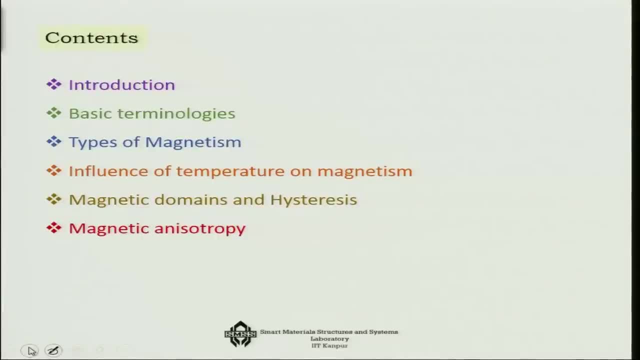 product development. So in this lecture we are going to give a small introduction to the magnetism 1 And basic terminologies, types of magnetism, influence of temperature on magnetism, magnetic domains and hysteresis and magnetic anisotropy. Now, as you know that magnet is always a very 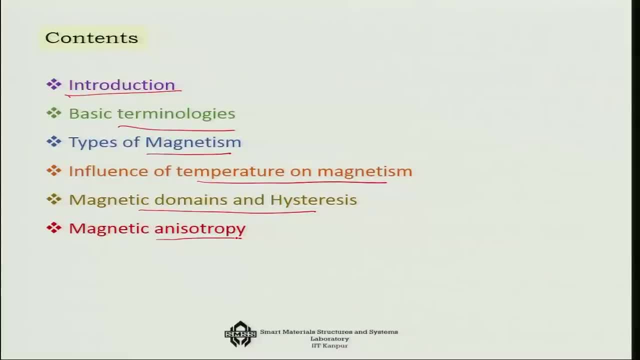 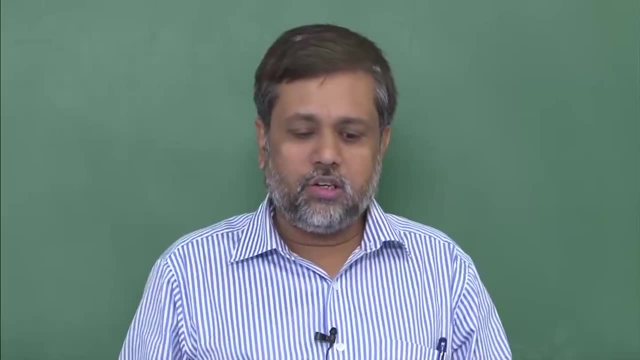 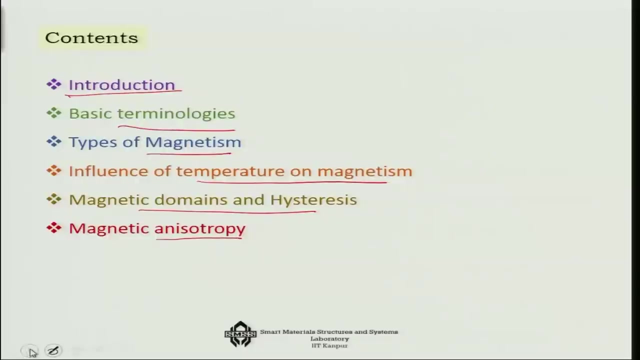 very mysterious material. People say that even Cleopatra used to take a bath in, you know, magnetic beads, thinking that it has some kind of correlationship with the longevity of a human being. It all happened because of that mystic force that you can see, a force, but the force is 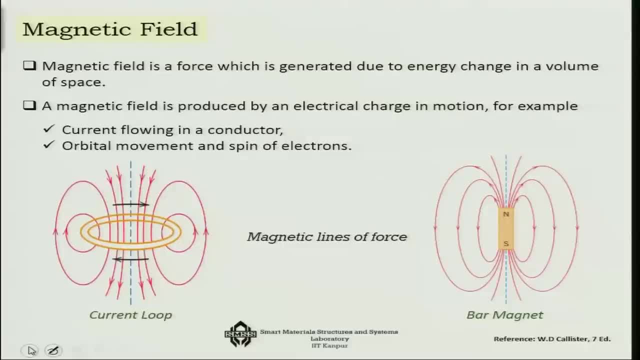 there which is working on you, So it is considered to be a very mystic force. So magnetic field is a force which is generated due to energy change in a volume of space, and this is produced by an electrical change in motion, For example, if there is a current flowing in a conductor. 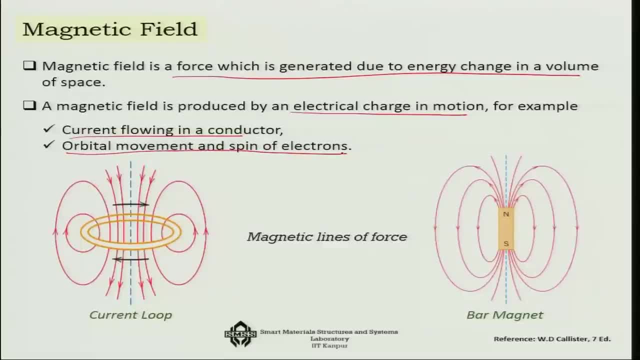 or orbital movement and spin of electron 2. So the magnetic field is a force which is generated by an energy change in a volume of space. So if there is a current loop, you will see that there are. you know the magnetic fields which are happening here. So in any current loop and if you consider a permanent, 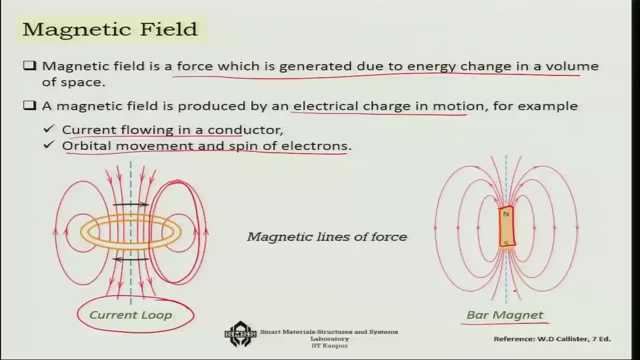 magnet, like a bar magnet for example, you would see that the magnetic field is generating from north and getting you know over at south. So that is how the magnetic lines of forces, the magnetic loops, are working on the system 3.. So basically, both you can have the magnetic field due to the intrinsic property of a material. 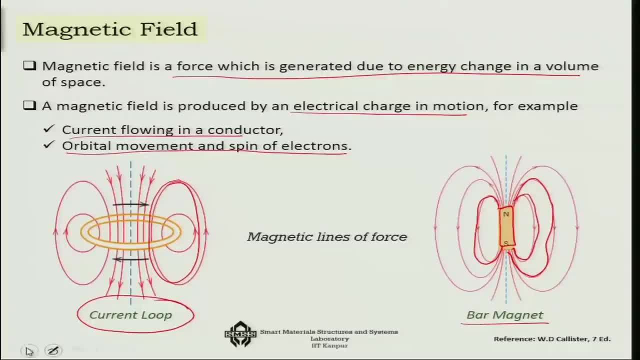 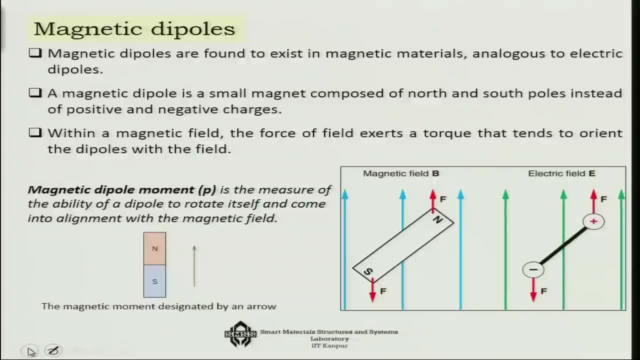 or you can have it by external electric field. in the system Now, similar to our electric dipoles, there are magnetic dipoles. In this case it is not a positive or a negative charge, but it is these north and the south pole. So magnetic dipoles are found to exist in. 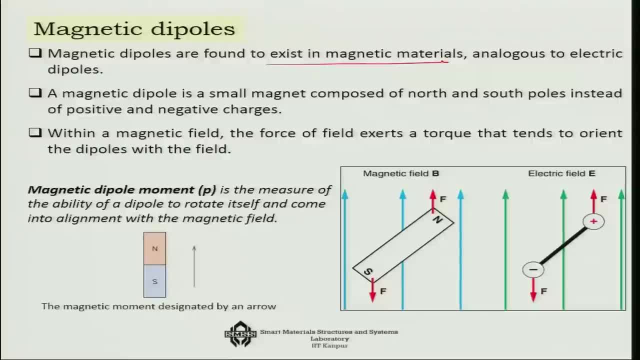 magnetic material. 3. So the försöory dipole are normallyphereỉ within a magnetic material, magnetic material, which are very much analogous to electric dipoles. And this magnetic dipole you can almost think like a miniature magnet, which 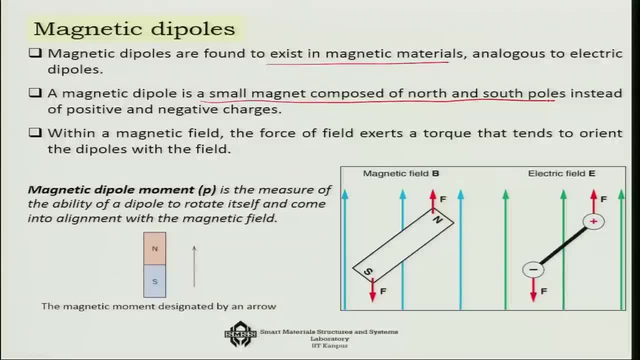 is composed of north and south poles instead of positive and negative charges Within a magnetic field. the force of field exerts a torque that tends to reorient these dipoles with the field. So it has. it is already. you know. for example, this is a breaks, a jet boil. 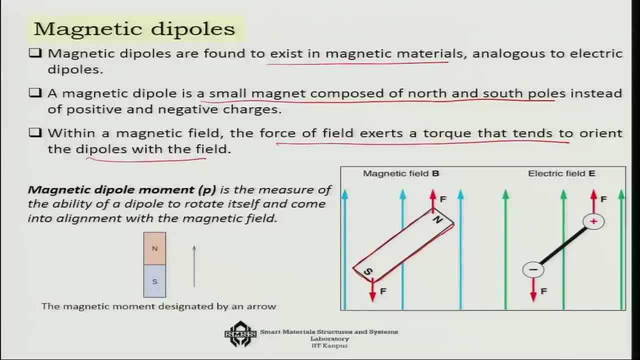 you can say that a, j pickup, 3. Si spolyo, 5.. So now what I am going takes up when remaining inside, the magnetic force is located within magnetic dipole, and then I am applying a magnetic field here, B, So this field will actually 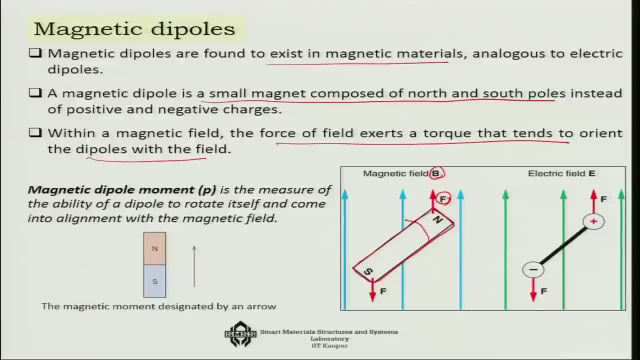 apply a force here, F, which will align, which will force it to align itself towards the direction of the magnetic field. Now it is, you know, very similar to the electric field based, you know, movement of the system. So magnetic dipole moment is the measure of the 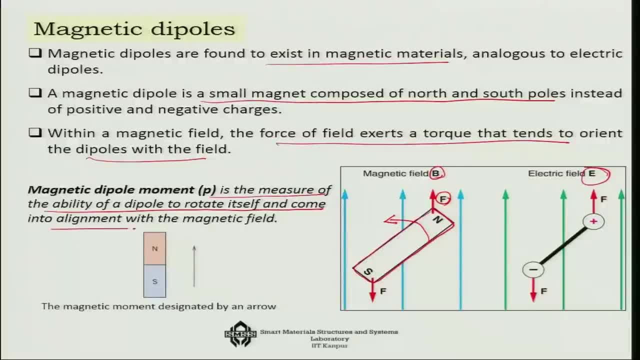 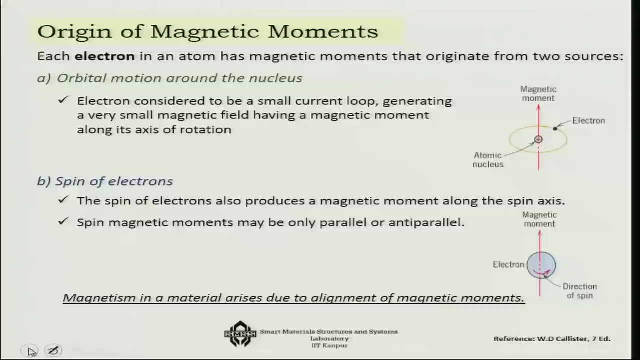 ability of a dipole to rotate itself and come into alignment with the magnetic field. Much the easily readily it can do, the more magnetic is, of course, the material, And we generally denote this magnetic moment by an arrow like this. Now there are. what are the origins of such magnetic moments? Well, there are two sources. 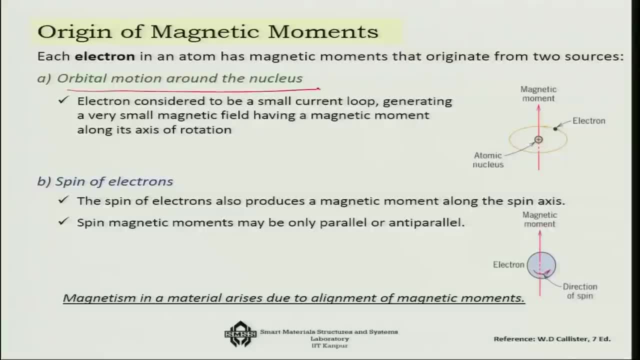 one is the orbital motion of electrons, Electrons around the nucleus, because they are like very, very small current loops, each electron orbiting along the nucleus of a atomic nucleus of a system. So each electron, during their motion, must generate a magnetic moment along its axis of rotation. a magnetic moment. 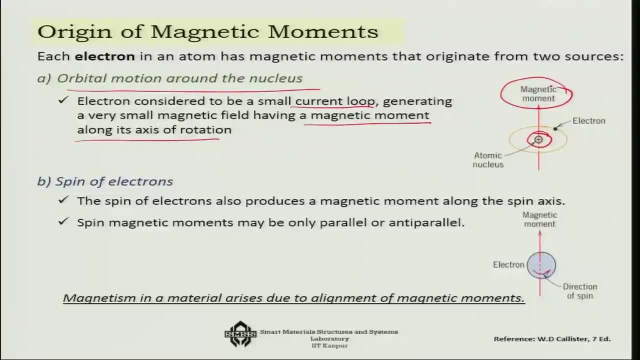 gets generated. Then there is the spin of electrons. this also produces a magnetic moment along the spinning axis. So this is like it is like each individual electron now which is spinning and that is creating a magnetic moment. So there are two motions that are there. right, You can? 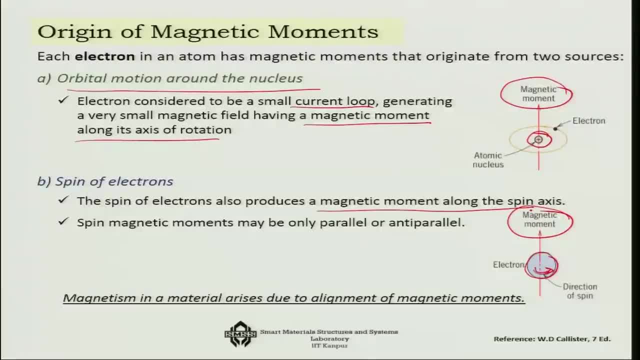 think of it very and much analogous to the motion of Earth around the Sun, That you have a motion of Earth around its own axis, which is like the spinning motion, and you have also the orbital motion. So the orbital motion generates one of the magnetic moment and the spinning motion generates another magnetic moment. both of these are 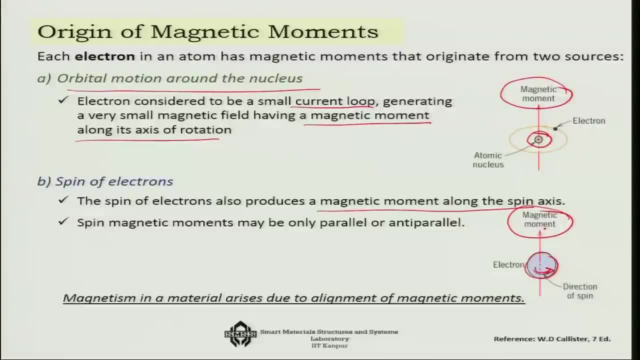 bound to happen. because? why? because the electrons carry the electric field. so the change of electric field, we know that is going to generate the magnetic field. So magnetism in a material arises due to alignment of the magnetic moments. that is in a macroscopic scale. we will talk about it. 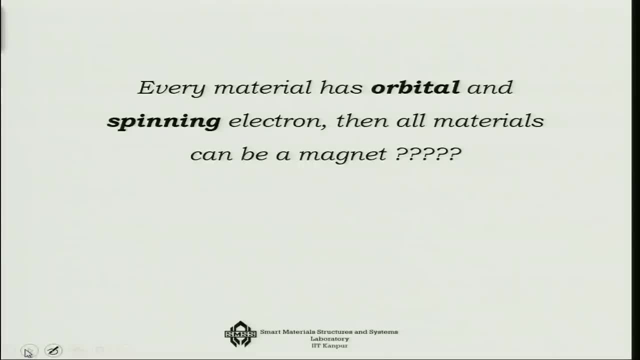 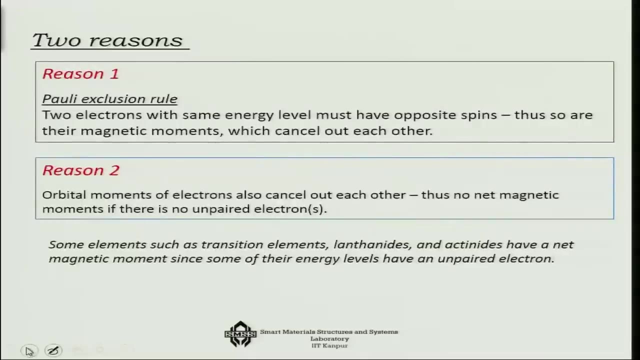 Now, every material has atoms, so it has orbital and spinning electron. then are all materials a magnet? the answer is no. so in the macroscopic scale it does not happen. So why it does not happen? two reasons. one reason is called the Pauli exclusion rule, which says that two electrons with same energy level- if it has, then it must have opposite. 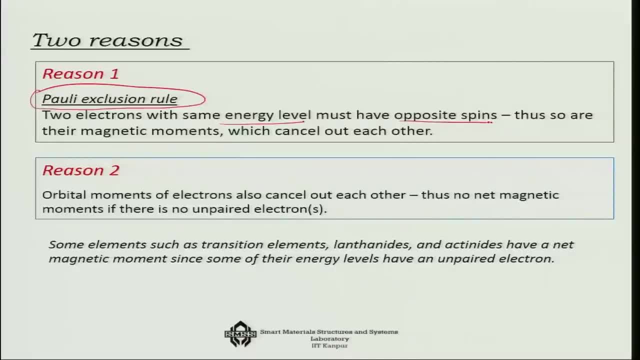 spins. So thus the their magnetic moments are going to cancel each other. so even though there are, if there are two electrons, they cannot be at the same spin. they will be in the opposite spin. as a result, the magnetic moment due to spinning is going to cancel. 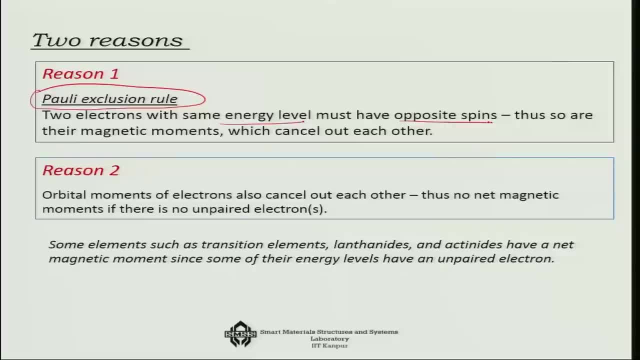 Then, as far as the orbital moment is concerned, that also cancel out each other. and there is no net magnetic moment if there is no unpaired electron. So the clue is that. So the clue is that If you have unpaired electron, only then this result will get manifested in the macroscopic. 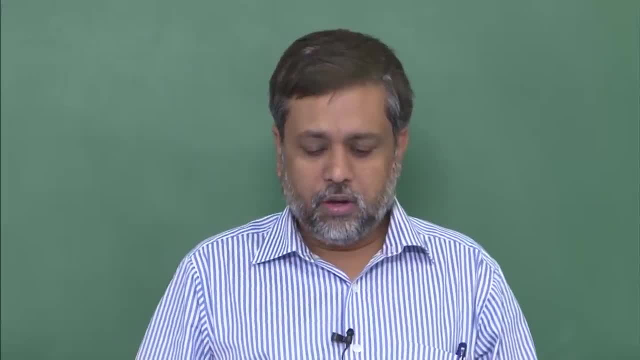 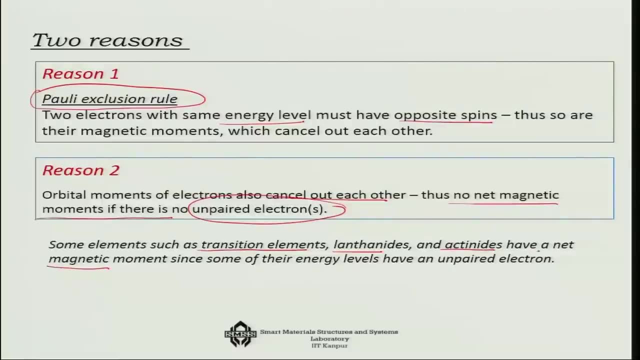 scale, otherwise they are going to cancel each other. Some elements, such as transition elements, lanthides and actinides. they have a net magnetic moment and some of their energy levels have an unpaired electron. that is why they show this kind of a magnetic moment. 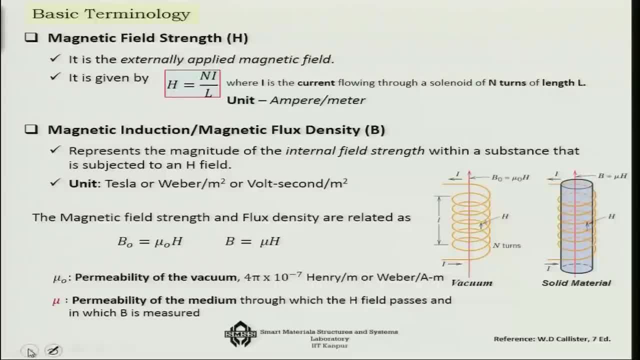 Now there are some basic terminologies With respect to these. you know magnetism. first thing is the magnetic field strength H. This is the externally applied magnetic field and it is generally described in terms of three parameters. number one is N, that is, total number of turns, and the length, that is L, on which. 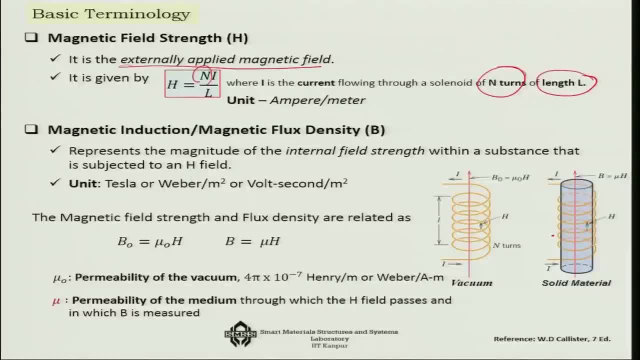 you are giving the turn. Suppose this is a solenoid, then the length of the solenoid. So this is the L and the current I. So if I increase the current in the coil I get more magnetic field. If I increase the length, then the magnetic field intensity comes down. 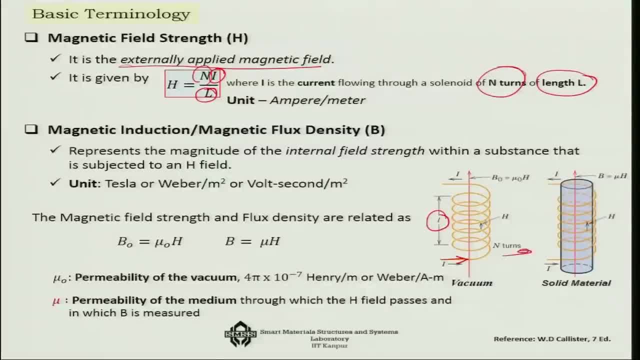 If I increase the number of turns, if I make it, you know, more dense, then I get actually more magnetic field out of the same length. So the number of turns plays also an important role. Now, next to H, H is fine. H equals to N, i over L that you know now and which has a unit of 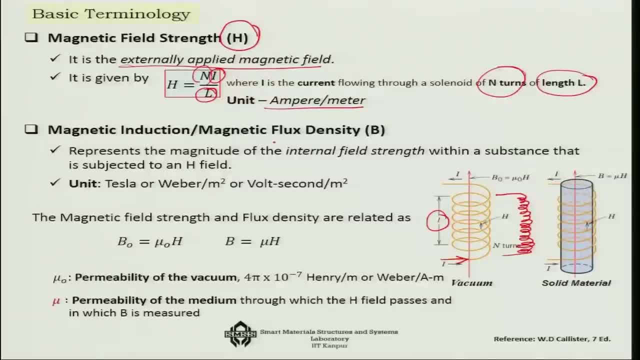 ampere per meter. next to that is the magnetic flux density B. This represents the magnitude of the internal field strength within a substrate that is subjected to an H field. So H is the field strength, So H is the field strength, But the density of that field, you know, which gets all around that density, is actually measured. 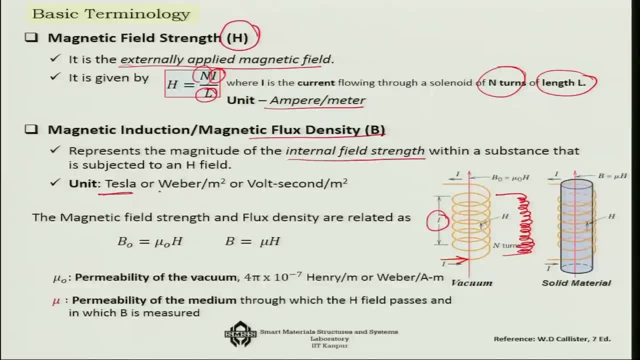 with respect to B, which has a unit of tesla or weber per square meter or volt second per meter square, The simple relationship here is: B equals to mu H. for vacuum, of course, it is mu 0 H. So where mu is now the permeability of the medium through the vacuum. 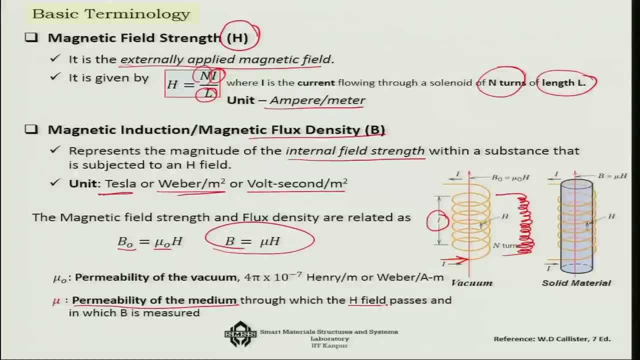 So this is the permeability of the medium through the vacuum. So this is the permeability of the medium through the vacuum. So this is the permeability of the medium. So this is the permeability of the medium through which the H field passes. 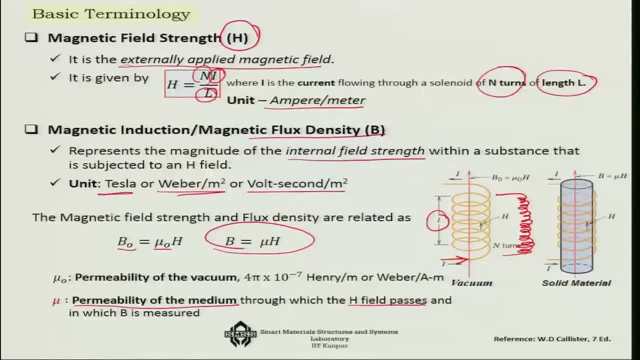 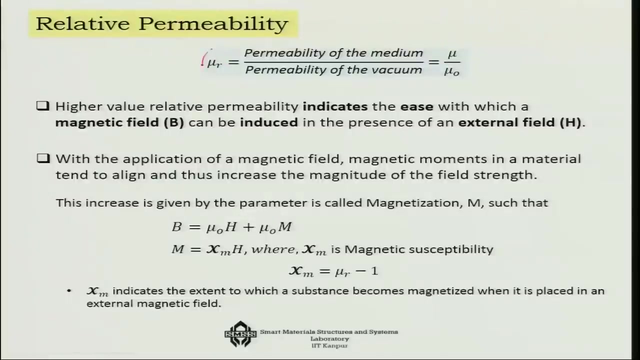 That means if the medium is more permeable, then with the same magnetic field strength you are going to get higher magnetic flux density. So permeability, mu, is a very important factor for us. Next, the permeability, of course, is measured here in terms of the relative permeability. 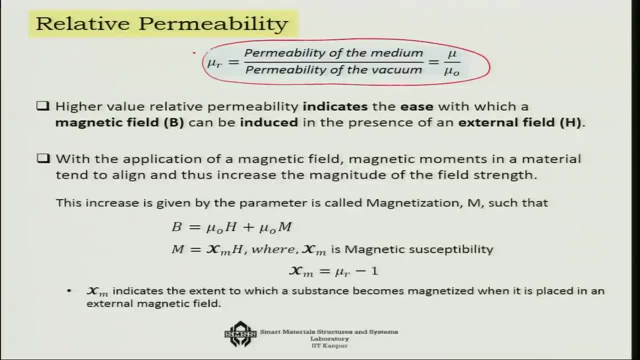 mu R, mu over mu 0. Okay, And higher the value of the, you know, permeability of the medium. then mu R is higher, which is fine with us. The other point is that there is, just like polarization, there is something called magnetization M which presents in the material. 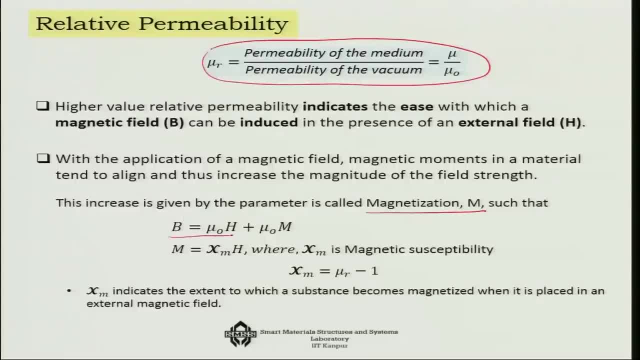 So, with respect to external field, the relationship was: B equals to mu 0, H. but what if the material is like you know, I told about like, Okay, You know, like an antonoids, etcetera. So there is a magnetization, that is there. 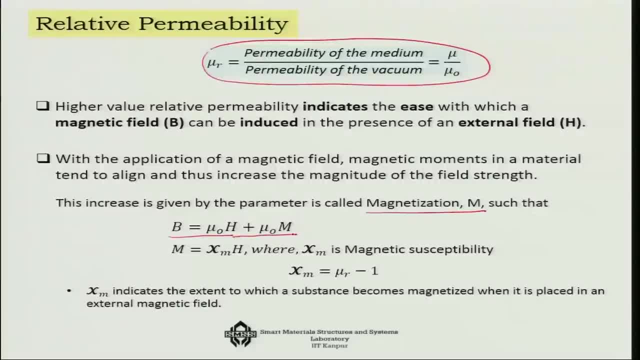 So you have to extend it to mu 0 plus mu 0 M, Where M is. once again, it can be expressed as a function of the field strength H, with the help of something called kappa M, where kappa M is the magnetic susceptibility, and this is mu R minus 1.. 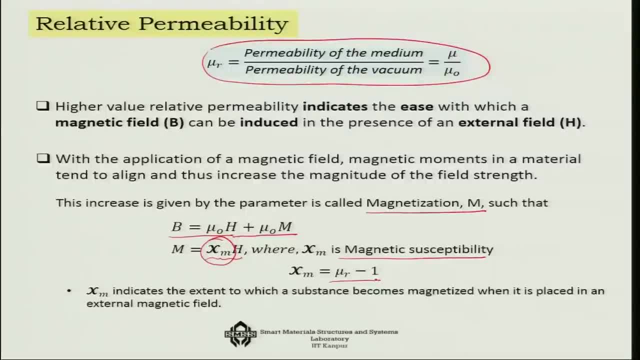 So, essentially, the property once again remains the same. So, essentially, the property once again remains the same. that is the relative permeability. So, essentially, the property once again remains the same. that is the relative permeability. that is the relative permeability because kappa also depends on the same. 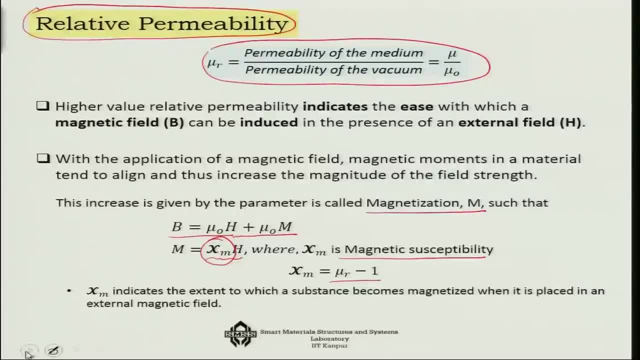 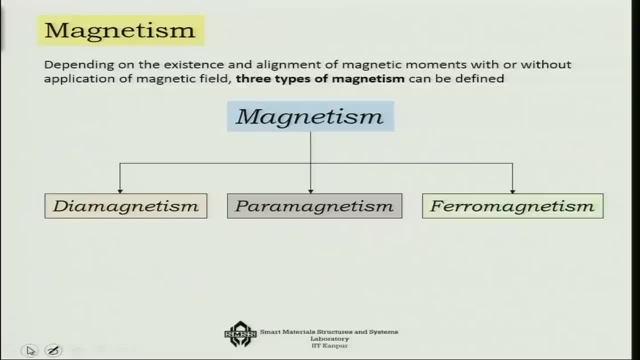 So this is how the magnetic field and the magnetic flux density are related to each other. Now let us talk about the manifestation of this magnetism on different materials. There are three types of magnetism that you will generally see. One is called diamagnetism, another is called paramagnetism, another is called ferromagnetism. 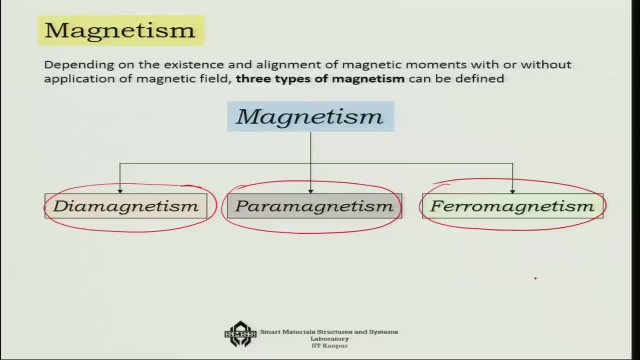 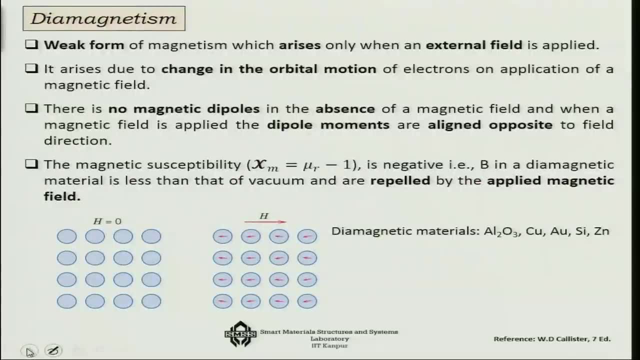 Of course, there are some or the other variation, but these are the basic three that you will see in a material. What is the diamagnetism? This is actually the weakest form of magnetism, which arises only when external field is applied. This arises due to the change in the orbital motion of electrons. on application of magnetic 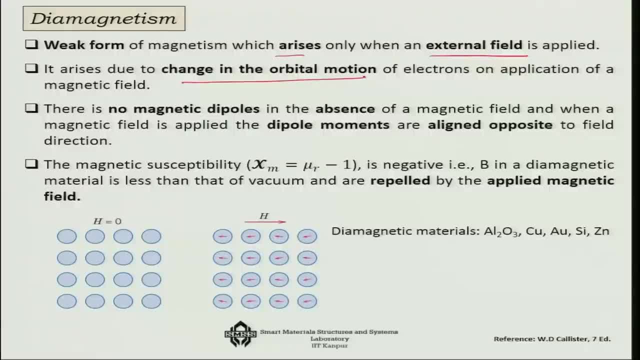 field, The orbital motion is going to get changed. There is no change. There are no magnetic dipoles in the absence of a magnetic field and when a magnetic field is applied, the dipole moments are aligned opposite to field direction, Like initially, there is no dipole moment and the moment you apply the magnetic field 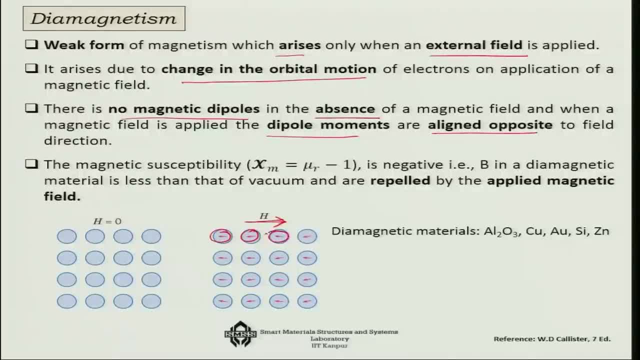 you are going to see that the dipole moments are coming. they are trying to balance opposite to the direction of the magnetic field. So this is the diamagnetic materials. The magnetic susceptibility, Of course, in this case is mu r minus 1, which is negative, and B in a diamagnetic material. 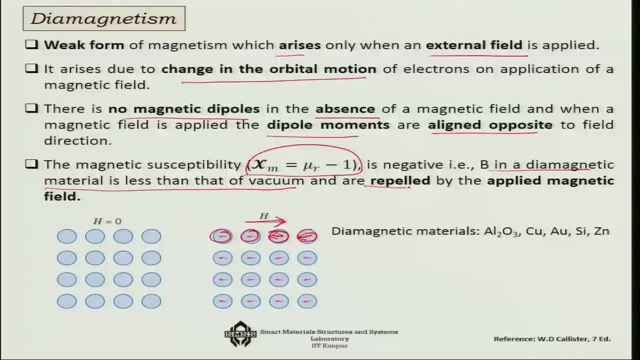 is actually less than that of vacuum and are repelled by the applied magnetic field. The examples of diamagnetic materials are like Al2O3, copper, gold, silicon, zinc, etc. One of the good use of diamagnetic materials is in terms of shielding from the electromagnetic 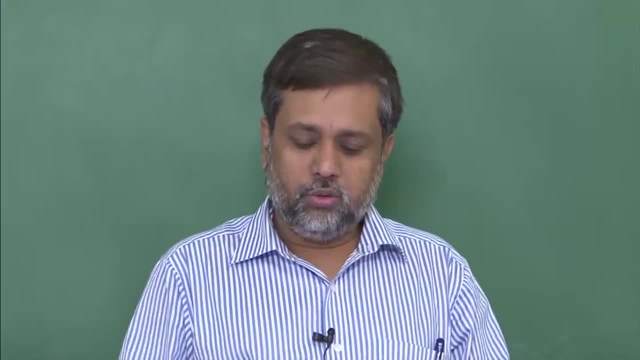 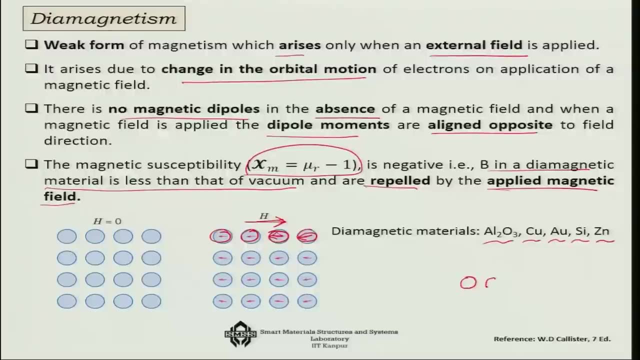 interactions. So we try to use this type of materials so that if you imagine that you have a series of such diamagnetic materials there as a protective coat and you have a very sensitive electronic circuitries that are there here, So some ICs are there- then if you apply a magnetic field, this immediately generates. 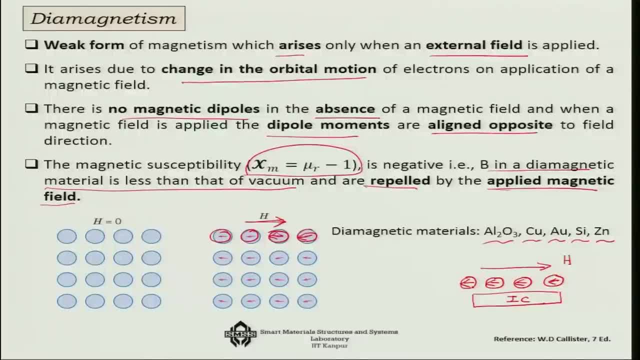 the opposite direction. So this is the direction of these, you know, magnetic dipoles, which will nullify this effect and, as a result, this IC will be saved from the effect of the magnetic field intensity. So that is how the diamagnetic materials are very, very useful as a protective coating. 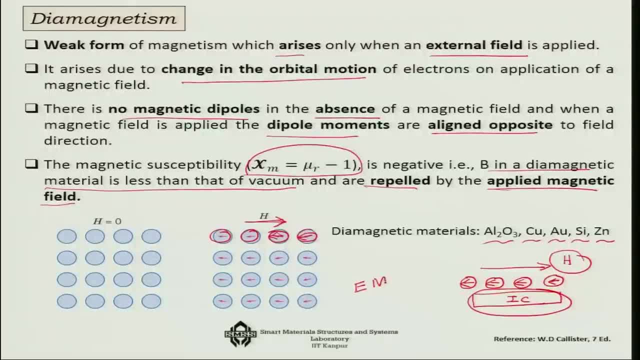 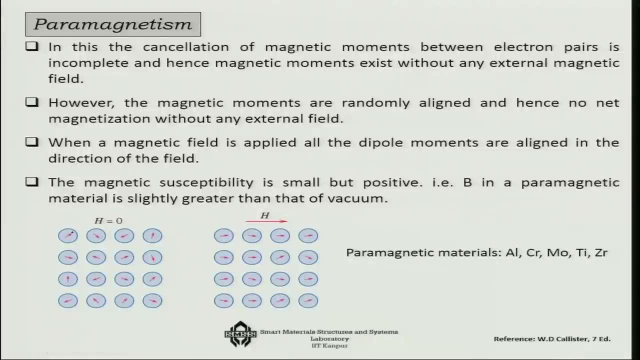 against electromagnetic interference. we call it EMI interference. Okay, Now paramagnetic materials. Okay, So in this, the cancellation of magnetic moments. this actually already has some unpaired electrons, since it has some internal magnetic moments, but in general they will not manifest. 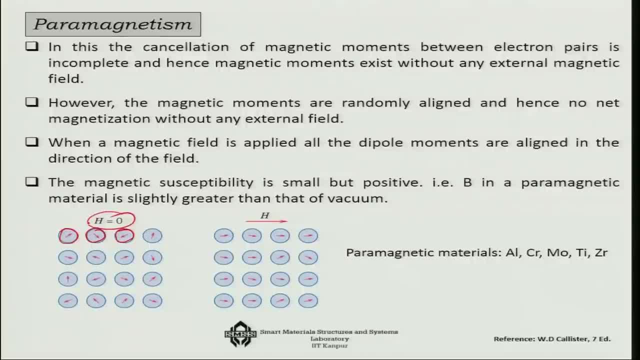 Why? Because they are random, so they are going to cancel each other. When a magnetic field is applied for paramagnetic material, they are going to align themselves towards the direction. So they are the traitors. They are going to align themselves towards the direction and hence they are slightly. 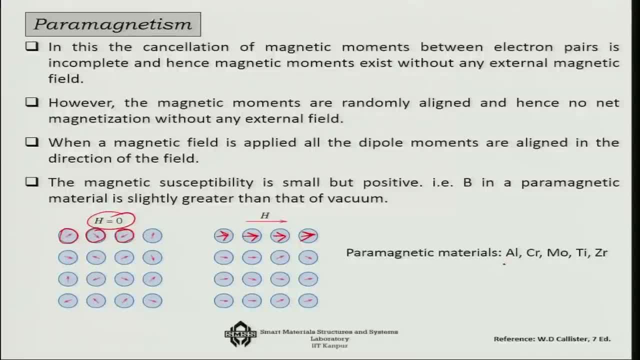 more magnetic than the diamagnetic materials. Examples are like aluminum, chromium, molybdenum. Examples are aluminum, chromium, molybdenum, titanium, zirconium, etcetera. So that is the paramagnetic materials. 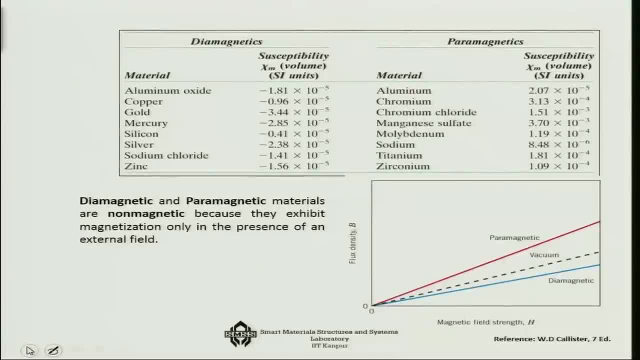 Now let us go to another group. Okay, So before we go to the ferromagnetics, this is like a chart which gives us the susceptibility of diamagnetic materials, because there we are measuring it in terms of the susceptibility, not the permeability. 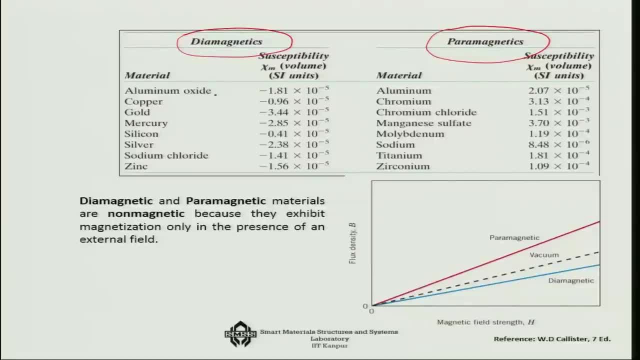 So it is like if you consider aluminum oxide among the diamagnetics, one of the highest in terms of susceptibility, Okay, Okay, So that is the gold, mercury, for example, then silver, for example, then there are other materials like sodium chloride, zinc, etcetera. 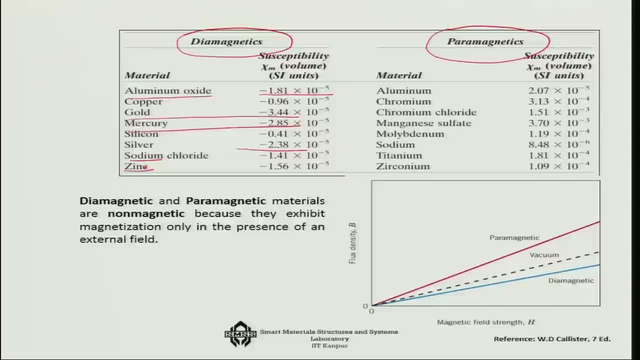 In terms of the paramagnetic materials. in terms of the paramagnetic materials, the one which will top the list is the sodium. as you can see, Some metals are also paramagnetic. Okay, Okay, Some metals are also paramagnetic, like you know. let us say aluminum, chromium. then there, 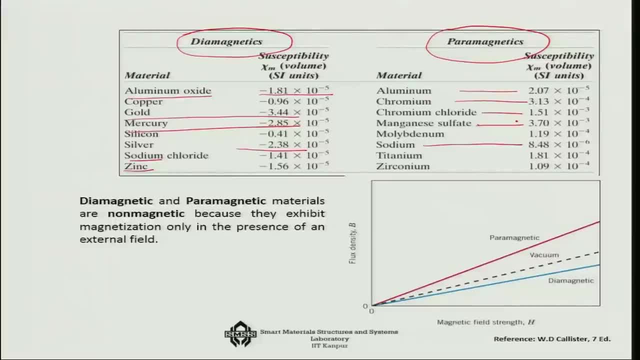 is some compounds like chromium chloride, magnesium, sulfate, molybdenum, titanium, zirconium, etcetera. So these materials are non-magnetic because they exhibit magnetization only in the presence of an external field. Okay, Okay. 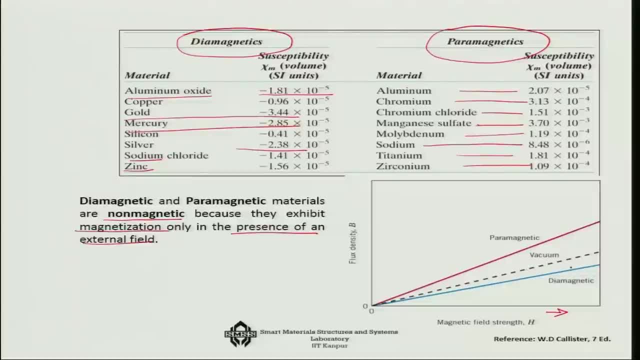 Okay, So the magnetic flux density increases. for the diamagnetic material it is still much lower than the vacuum, and for the paramagnetic material it increases, you know, slightly with the help of the magnetic field H. So that is the diamagnetic and the paramagnetic material. 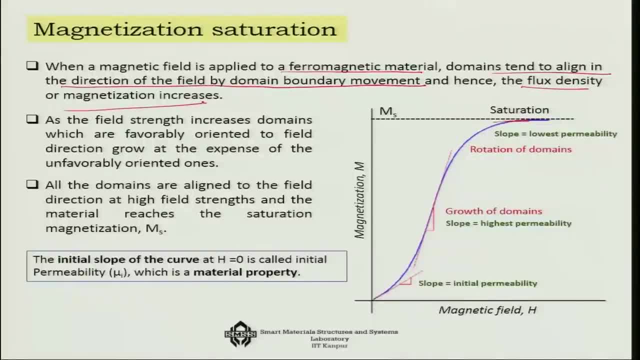 density or magnetization increases. This is just what I wanted to show you earlier. that you know. suppose this is your initial permeability And then suddenly there is a growth of domains. that means you know all these domains that you have seen in a volume. suppose you have some such domains. the domains are not stationary. 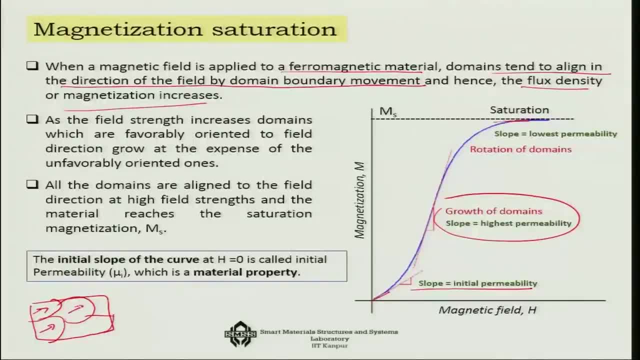 in nature. So each domain size are going to increase with respect to the magnetic field, So you may become more chunk and bigger and bigger. So this is the growth of domains, So the magnetization also is increasing, but beyond a certain point the entire you. 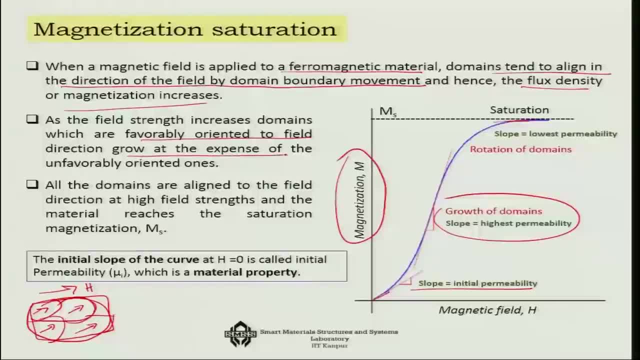 know, all the domains are favorably oriented to field direction grow at the expense of the unfavorably oriented ones. that is this point. And then, once domains are aligned to the field direction at high field strengths and the material which is the saturation magnetization M s, then, you know, this whole activity becomes. 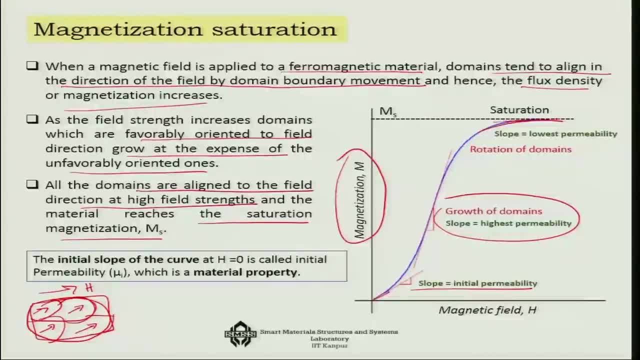 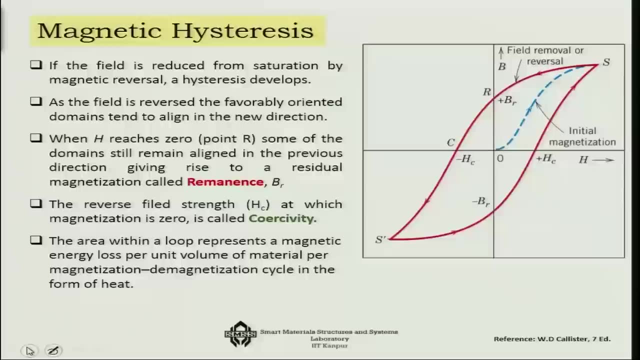 once again very much get saturated. So the there is no need change in magnetization anymore with respect to the change of the magnetic field. So that is how we get that- a famous S curve in it. There is one interesting thing: if you change the direction of magnetization, then what happens? 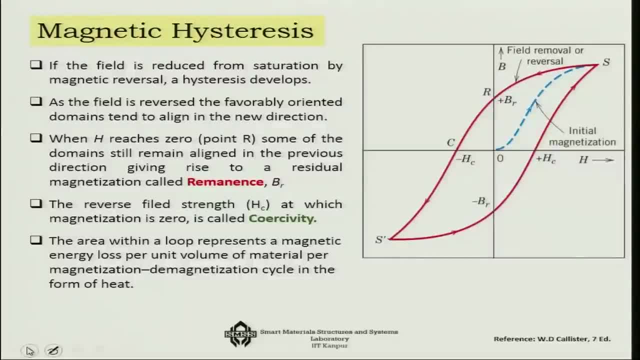 So if the field is reduced from saturation by magnetic reversal, there is a hysteresis that would develop. As the field is reversed, The favorably oriented domains tend to align to the new direction. When h reaches 0, some of the domains still remain aligned in the previous direction. 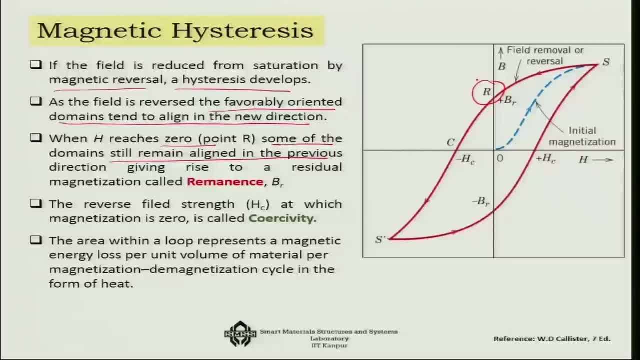 This gives you a magnitude of remnance. this gives you a residual magnetization called remnance. The reverse field strength at which the magnetization becomes zero is called the quercivity. quercivity is the reverse field strength of the magnetic field. 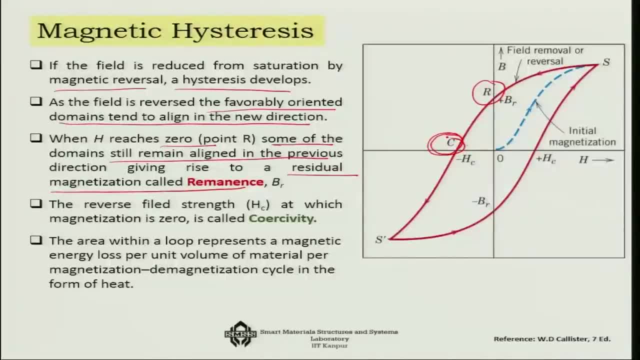 magnetization becomes 0.. There are two important things in magnetic hysteresis. One is called, as I told you, the remnants. That means when you are reversing the magnetic field, you will still find that some domains have not really, you know, aligned themselves or it is still keeping this alignment that 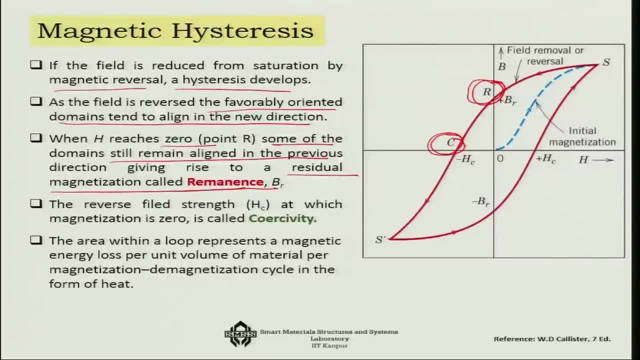 is what is the remnants there? And then when you are having already a negative- you know- magnetic field, you will still find that suddenly it will become 0, so that is the versivity: when the you know, the magnetization will become 0. 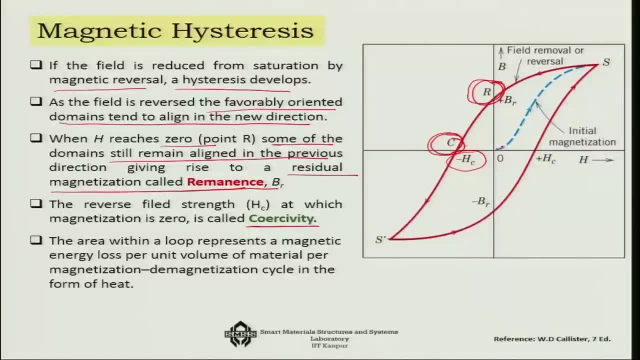 The other thing is that this all, so this is the initial root, and then you are reversing the magnetic field. So up to this you are increasing and then you are reversing it. and as we are reversing it, we are going down like this, And when you are again reversing the magnetic field, it is coming in a different line, meaning: 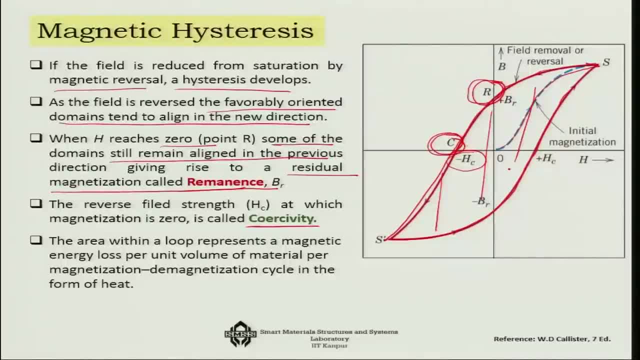 thereby you will have an area inside which is the hysteresis of the- you know, magnetic hysteresis. So there is some amount of energy which will be basically lose. you are losing that, that is what. So the hysteresis is signified by this hysteresis, and that happens in every magnetization, demagnetization. 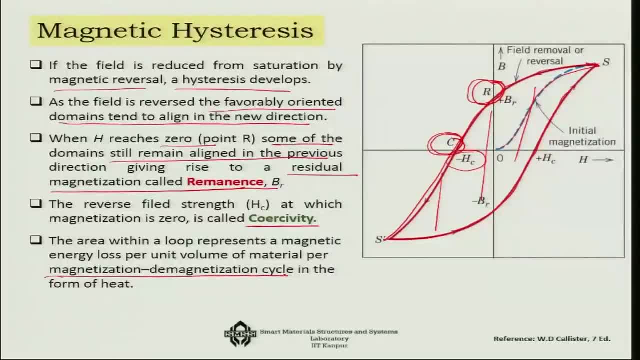 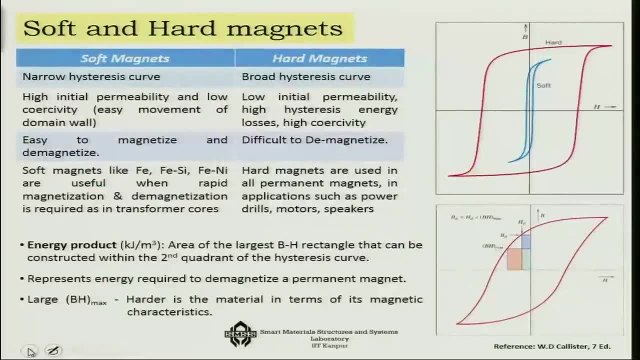 cycle. Where does the energy go? Well, it goes for heat energy, for example, acoustic energies, etcetera. that is the magnetic hysteresis in the system. There are two different types of magnets that we categorize in terms of this hysteresis. 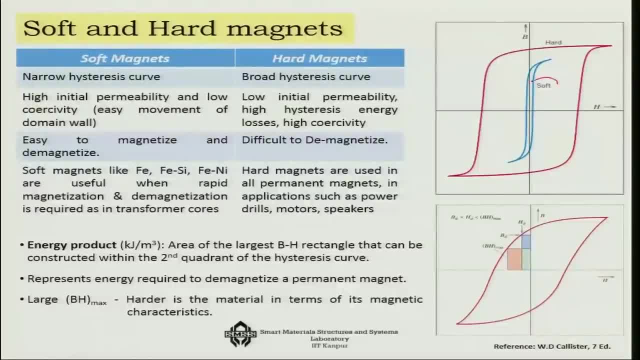 One is called soft magnet, which has a narrow hysteresis curve, and another is a hard magnet. So the comparison is that indeed soft has a narrow hysteresis curve. it has high initial permeability and low coercivity, that is, easy movement of domain wall. 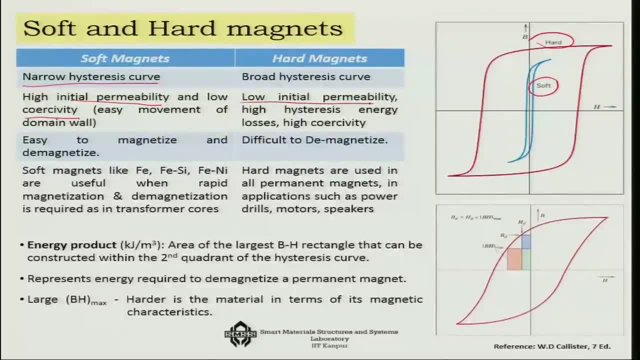 And in terms of hard magnet, is a low initial permeability, high hysteresis, energy losses, but high coercivity. also we look at it, it has a high coercivity. soft magnets are easy to magnetize and demagnetize, But hard magnets are difficult to demagnetize. 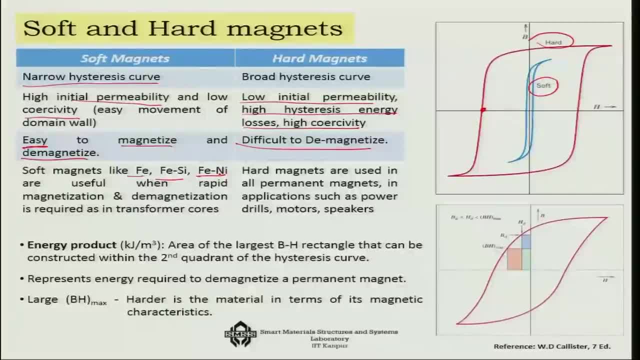 Soft magnets like iron, iron-silicon, iron-nickel. they are useful when rapid magnetization and demagnetization is required in a transformer core, for example. Hard magnets, on the other hand, they are used in all permanent magnets in application such 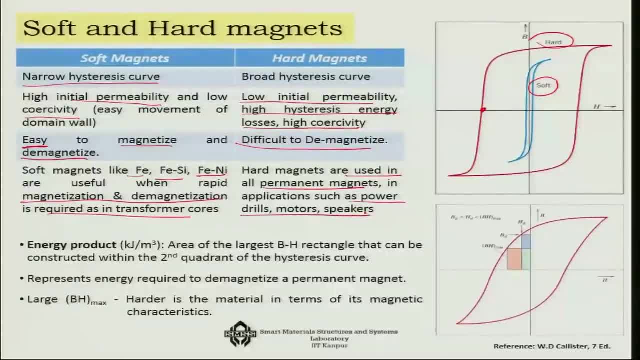 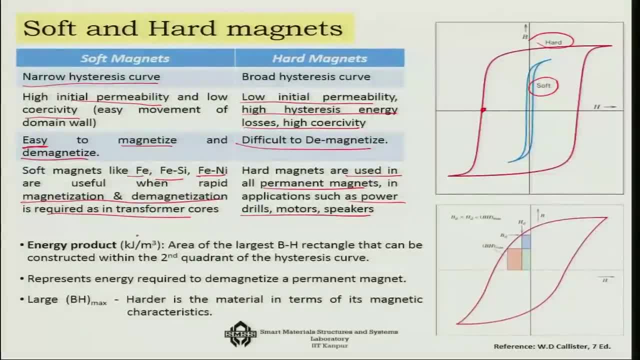 So the coercivity is very high. So the coercivity is very high. So the coercivity is very high because these all such things are not at theる, The energy product, which is, you know, in terms of kilo joule per meter cube. 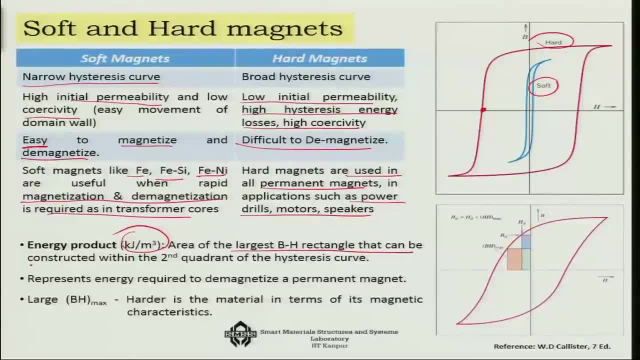 That is the area of the largest BH rectangle that can be constructed within the second quadrant of the hysteresis curve. This is the second quadrant of the hysteresis curve, So this is one of the measure, that is, the what is the largest, you know, BH rectangle. 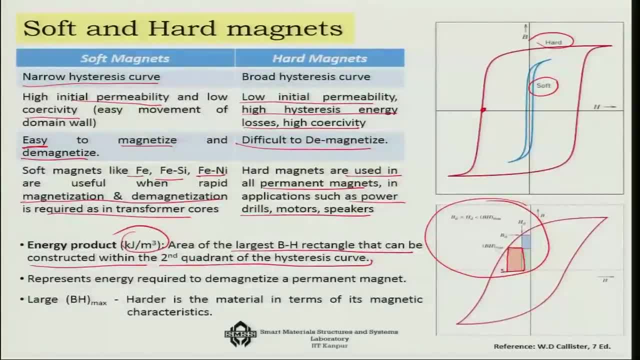 that you can fit here. that is the measure like this one, that is the measure of the hysteresis. hysteresis, This represents energy required to demagnetize a permanent magnet. based on that, you can. So larger the BH max, harder is the material in terms of its magnetic characteristics. 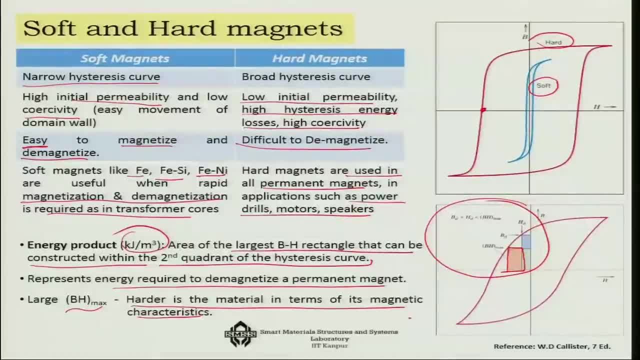 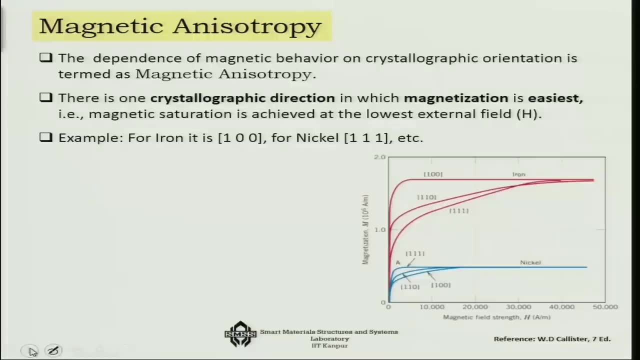 So you can. you know you all already we have talked about mu, the magnetic field permeability. Now we have a new one, that is the BH max, which is important in terms of categorization of soft and hard magnets. Next is magnetic anisotropy: The dependence of the magnetic behavior on 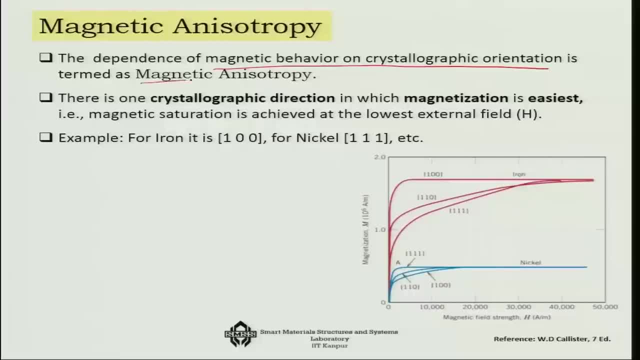 crystallographic orientation is termed as the magnetic anisotropy Because, as you know, that not all the directions it easy for the magnetization. So the crystallographic direction in which magnetization is easiest, that means magnetic saturation, is achieved at the lowest.